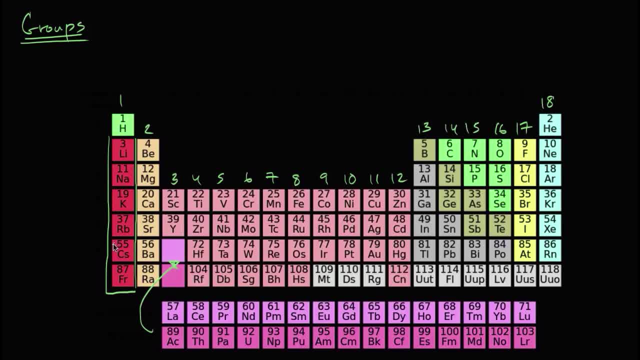 They tend to have the same number of valence electrons and valence electrons and electrons in the outermost shell tend to have the same number of electrons. in the outermost shell. They tend to coincide, although there's a slightly different variation: The valence electrons. these are the electrons. 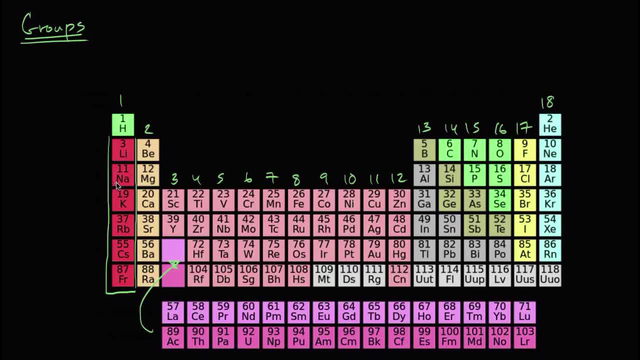 that are going to react, which tend to be the outermost shell electrons. but there are exceptions to that and there's actually a lot of interesting exceptions that happen in the transition metals in the D block, But we're not going to go into those details. 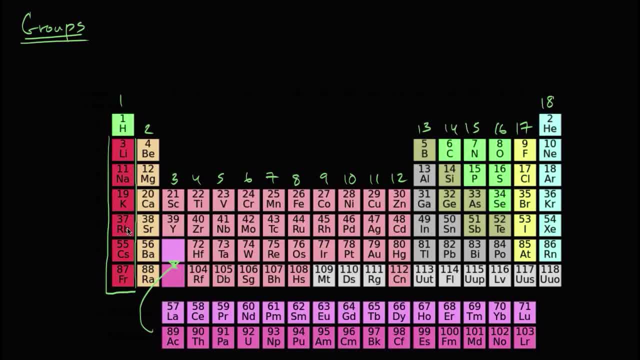 Let's just think a little bit about some of the groups that you will hear about and why they react in very similar ways. So if we go at group one And hydrogen is a little bit of a strange character, because hydrogen isn't trying to get to eight valence electrons- 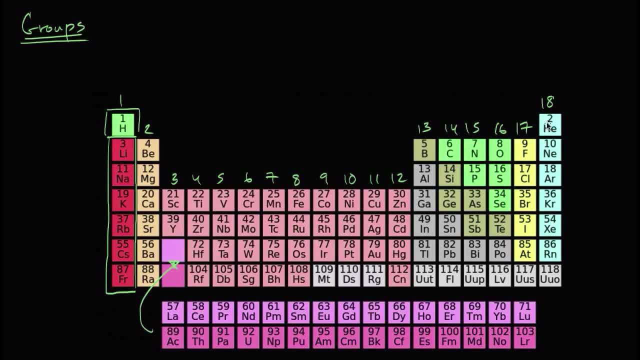 Hydrogen in that first shell just wants to get to two valence electrons, like helium has, And so hydrogen is kind of it doesn't share as much in common with everything else in group one as you might expect for, say, all of the things in group two. 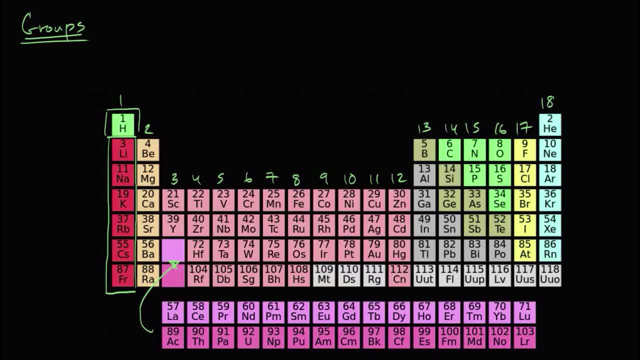 Group one. if you put hydrogen aside, these are referred to as the alkali metals, And hydrogen is not considered an alkali. It's an alkali metal. So these right over here are the alkali alkali metals. Now why do all of these have very similar reactions? 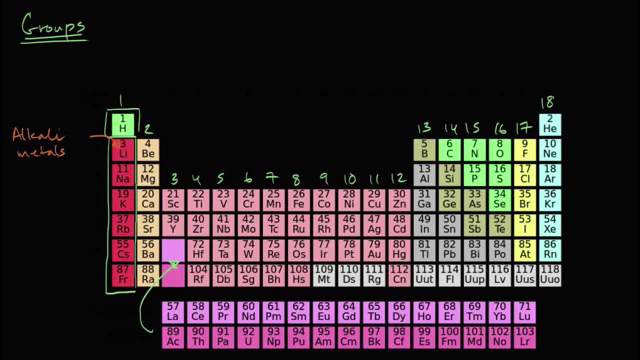 Why do they have very similar properties? Well, to think about that, you just have to think about their electron configurations. So, for example, the electron configuration for lithium is going to be the same as the electron configuration of helium, of helium. 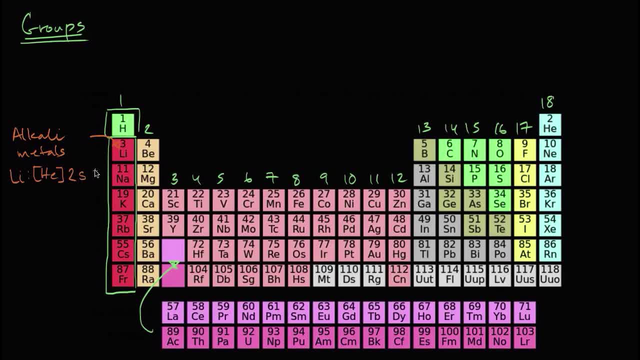 And you're going to go to your second shell, 2s1.. It has one valence electron. It has one electron in its outermost shell. What about sodium? Well, sodium is going to have the same electron configuration as neon. 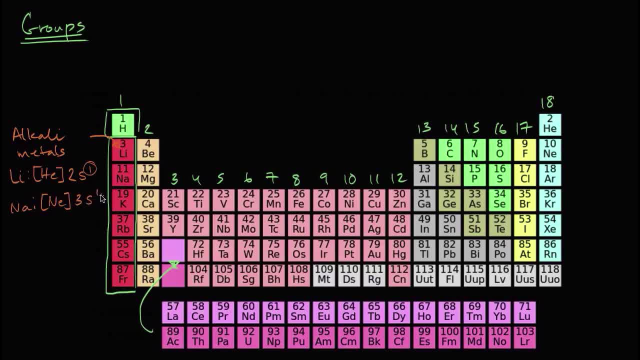 And then it's going to go 3s1.. So once again it has one valence electron, one electron in its outermost shell. So all of these elements in orange right over here, they have one valence electron. 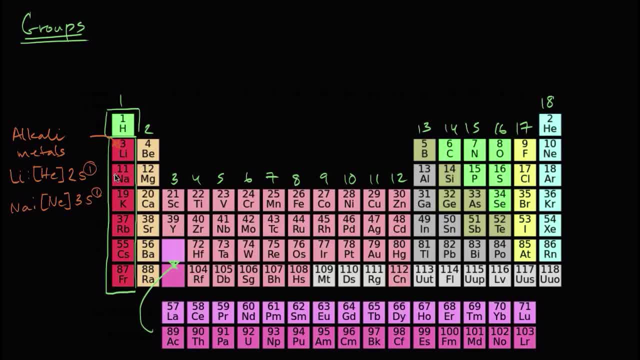 And they're trying to get to the octet rule, this kind of stable nirvana for atoms, And so you can imagine- is that they're very reactive And when they react, they tend to lose this electron in their outermost shell, And that is the case. 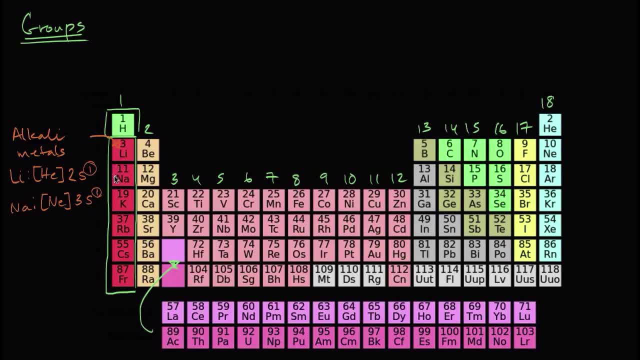 These alkali metals are very, very reactive And actually they have very similar properties. They're shiny and soft And actually, because they're so reactive, it's hard to find them where they haven't reacted with other things. Well, let's keep looking at the other groups. 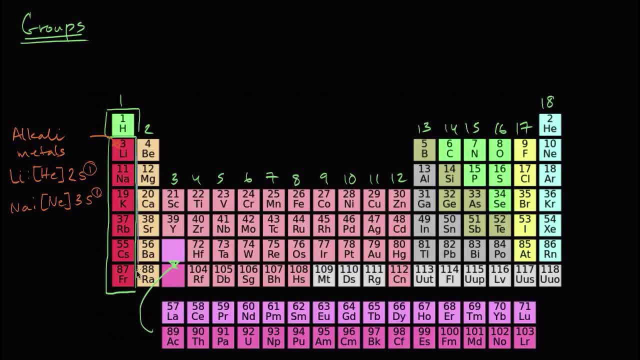 Well, if we move one over to the right, this group two right over here. these are called the alkaline earth metals- Alkaline alkaline earth metals- And once again they have very similar properties And that's because they have two valence electrons. 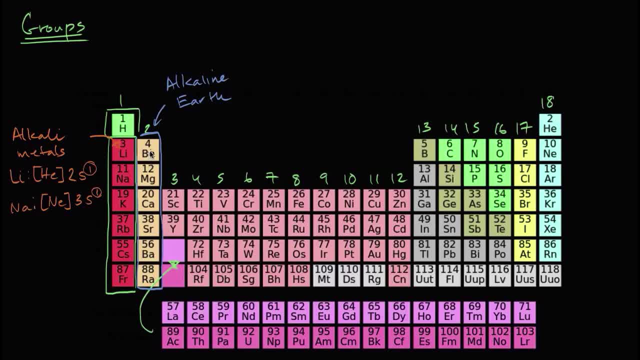 two electrons in their outermost shell And also for them not quite as reactive as the alkaline metals- But let me write this: alkaline earth metals, But for them it's easier to lose two electrons than to try to gain six, to get to eight. 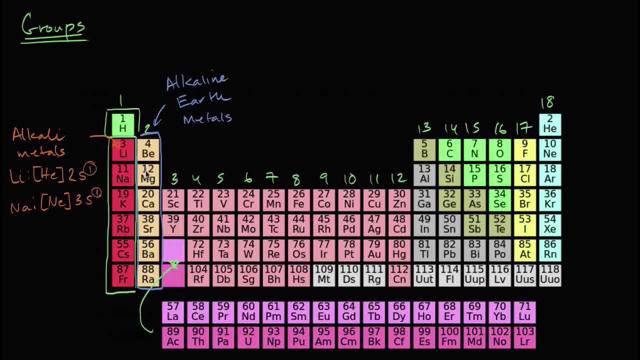 And so these tend to also be reasonably reactive, And they react by losing those two outer electrons. Now something interesting happens as you go to the D block, And we studied this when we looked at electron configurations. But if you look at the electron configuration for, say, 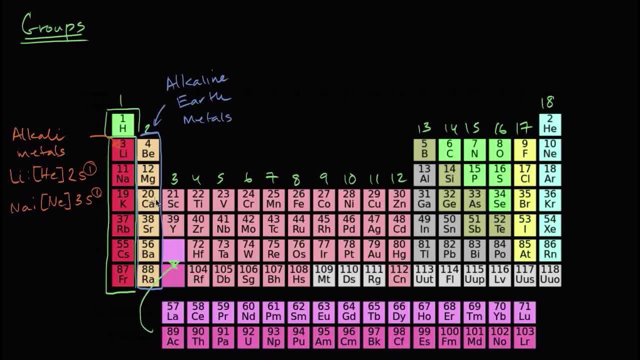 scandium, right over here the electron. let me do it in the electron configuration for scandium. So scandium, scandium's electron configuration is going to be the same as argon. It's going to be argon, The Aufbau principle would tell us. 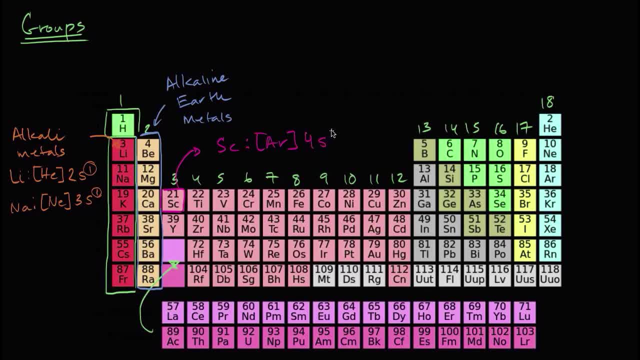 that the electron configuration, we would have the 4s2, just like calcium, But by the Aufbau principle we would also have one electron in 3D, So it would be argon 3D1, 4s2.. 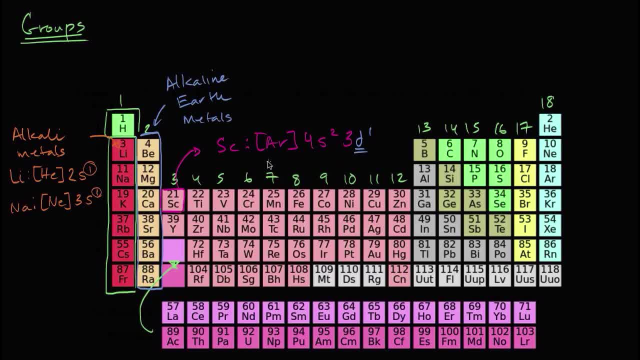 And to get things in the right order for our shells, let me put the 3D1 before the 4s2.. And so when people think about the Aufbau principle, they imagine all of these D block elements as somehow filling the D block. 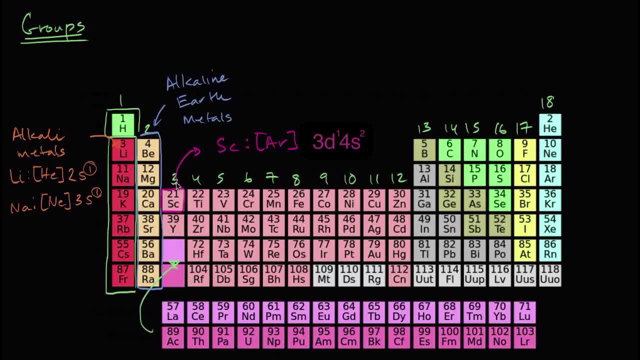 Now, as we know in other videos, that's not exactly true. But when you're conceptualizing the electron configuration it might be useful. Then you come over here and you start filling the P block. So, for example, if you look at the electron configuration,